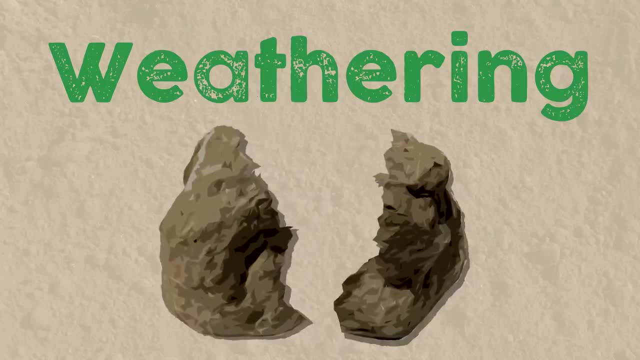 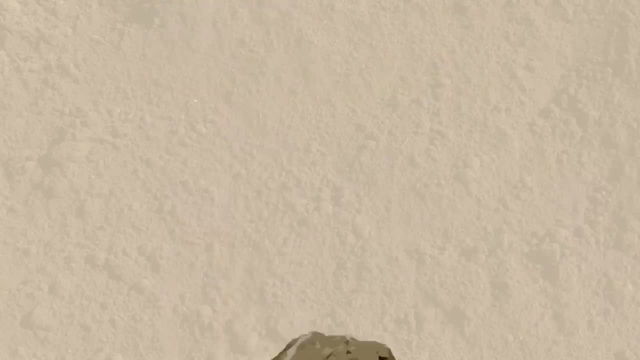 Weathering is the breaking of rocks into smaller rocks, either by a physical or a chemical process, And erosion is when these smaller rocks are carried away from the bigger parent rocks, usually by wind or water. Depending on the size of the weathered rock, it can either be considered a clay, a silt or a sand. 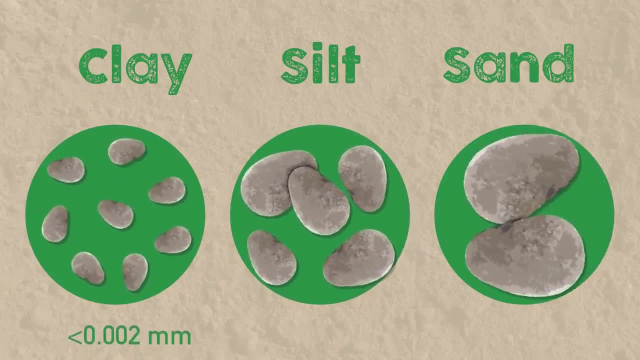 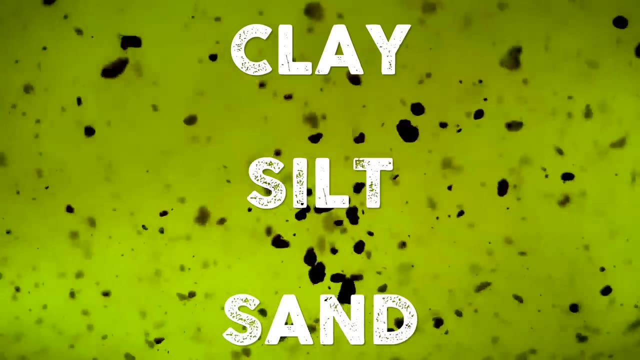 with anything bigger being gravel. Out of these three, though, clay is by far the smallest, while sand is the biggest, and silt is somewhere in between. Together, these three sizes of weathered and eroded rock make up soil, And 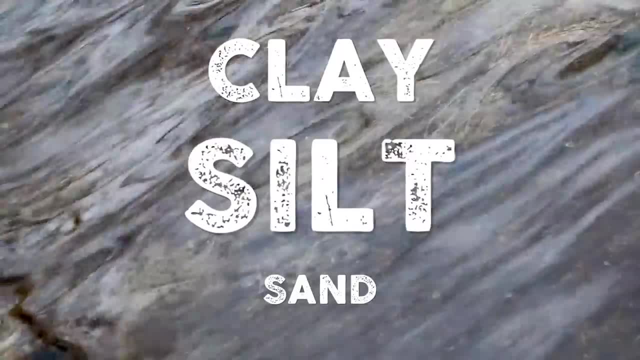 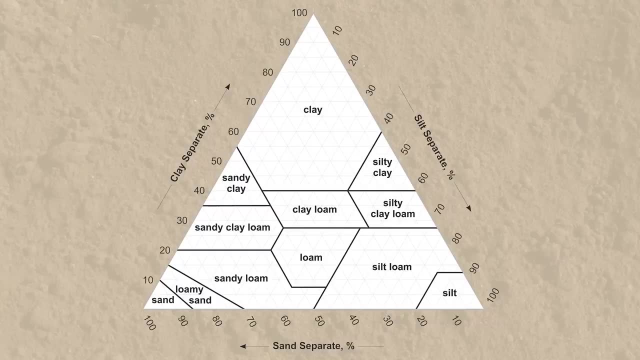 depending on the ratio of these three different sizes of particles, the soil will have different properties. There's this nifty graph to help figure out what you have, based on the soil's composition. So if a soil is 25% sand, 40% silt and 35% clay, it's considered clay alone. 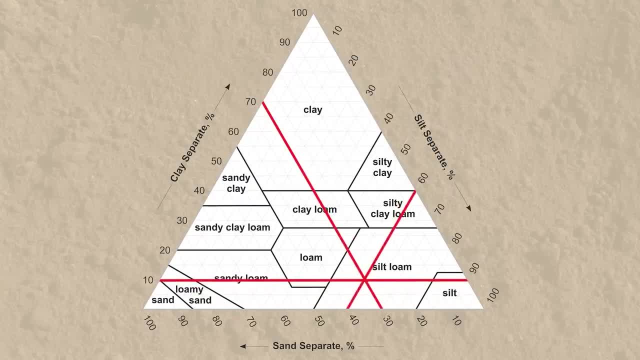 If it's 10% clay, 40% sand and 50% sand and 50% silt, it's silty loam. We could do this all day, And all these different combinations have differing properties. In most cases, however, loam is what you want your soil to be, as it's best for most types of plants to grow in. 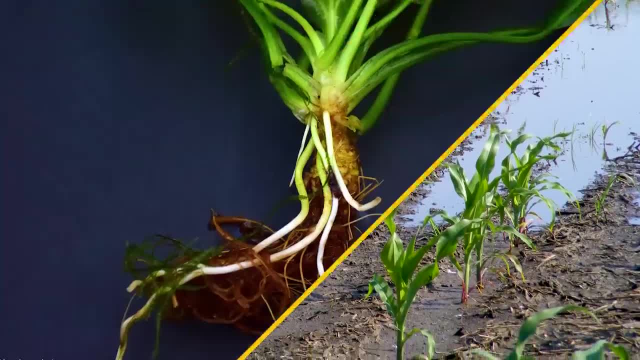 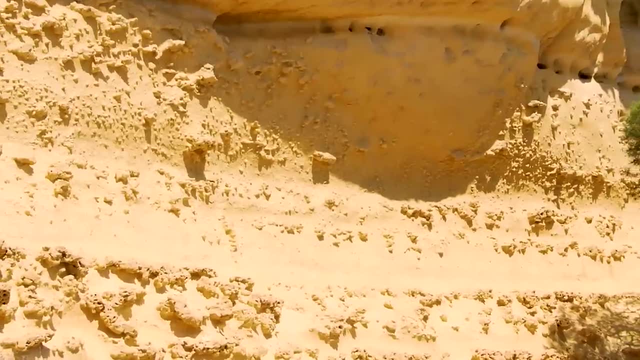 If a soil is more clay-like it will retain more water, but plant roots will have difficulty growing through it. If it's more like sand, it'll be worse at holding water but easier for roots to grow in Again. silt is kind of just the in-between and has characteristics of each extreme to lesser degrees. 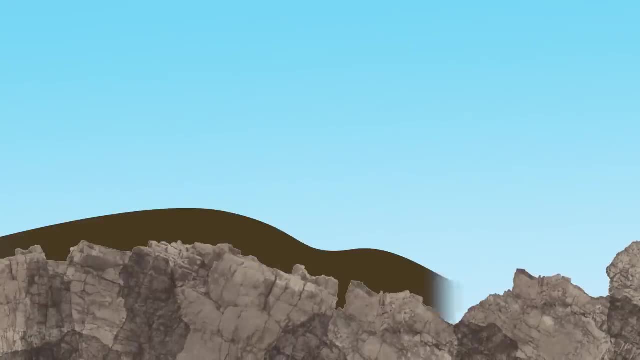 Overall, you want a good balance of each one. As these soils settle on top of each other, you'll find that the soil will be more silty and the roots will be more silty. As these soils settle on top of bedrock, they form into layers, called horizons. 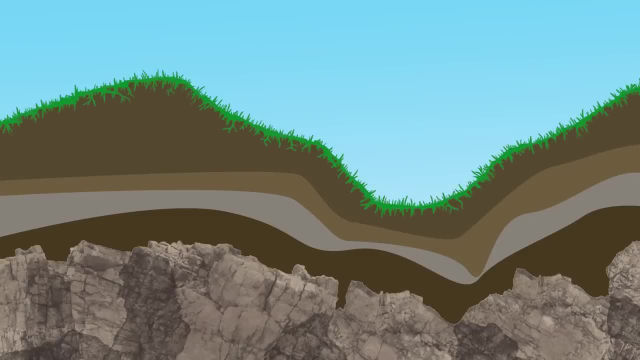 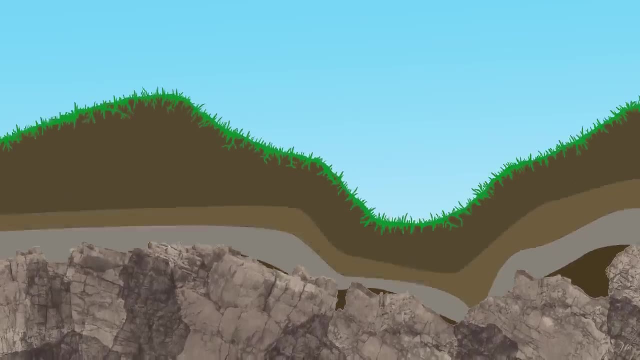 This process takes place over many thousands of years, as rock is weathered and eroded and moved from one place to another- And of course, things like this are never exact, as nature tends towards randomness- But for most places, five distinct horizons can typically be observed. 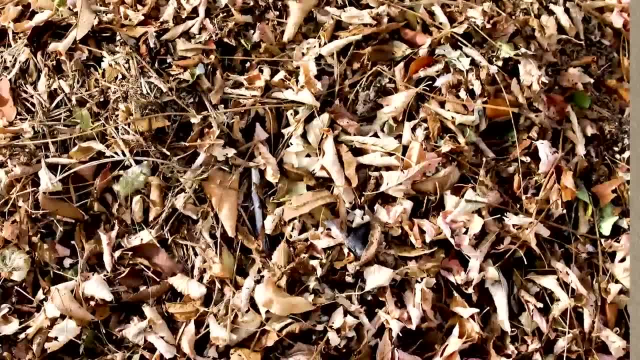 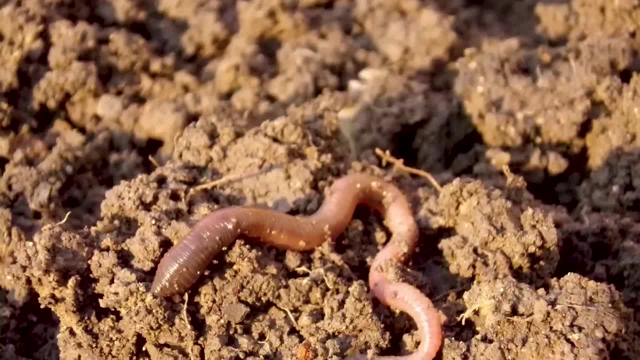 The uppermost is the O horizon- O for organic, and this is where most of the dead plant matter called detritus is. Then there's the A horizon. that's where the real surface soil is sometimes called the bio mantle, because this is also where most soil organisms reside. The B is the 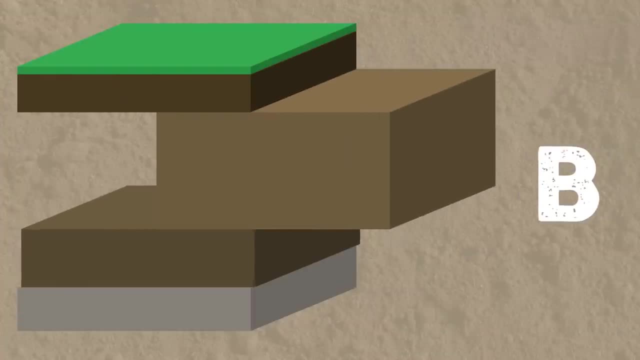 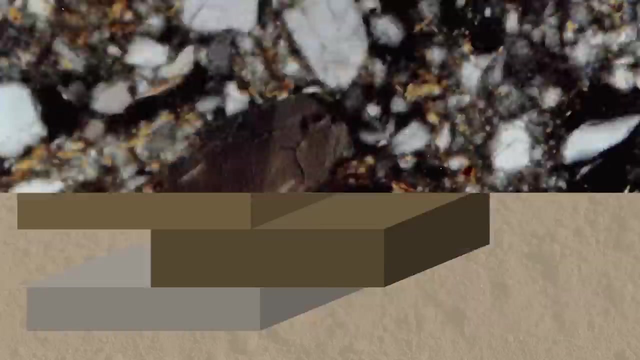 subsurface and usually is the furthest plant roots would go for soil. The C horizon is where the bedrock is slowly degrading into soil, so it's mostly large rocks and gravel with some soil in between. Then the R horizon: R for rock. 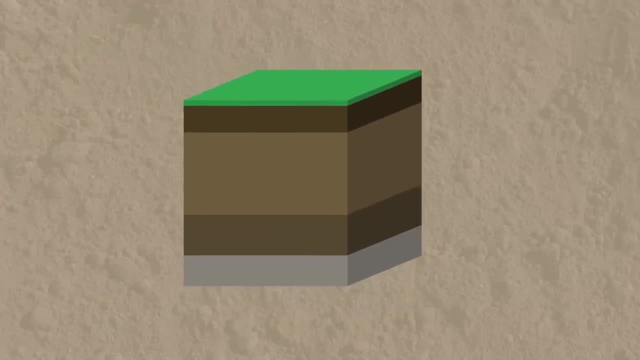 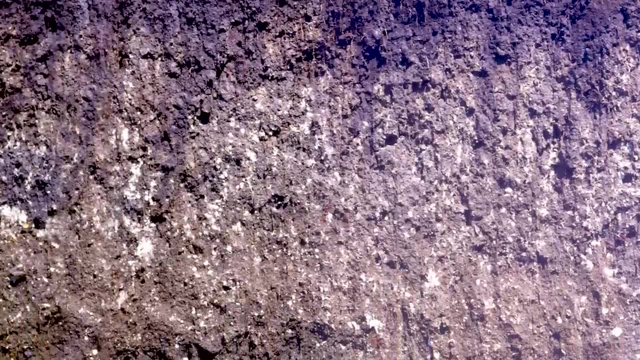 It's just rock. Sometimes, if there's a lot of soil leaching, an E horizon will develop. This is where sand and silt are deposited, while clay will continue further down into the B horizon, forming a thin light layer between the A and the B. And now here's where things get fun. 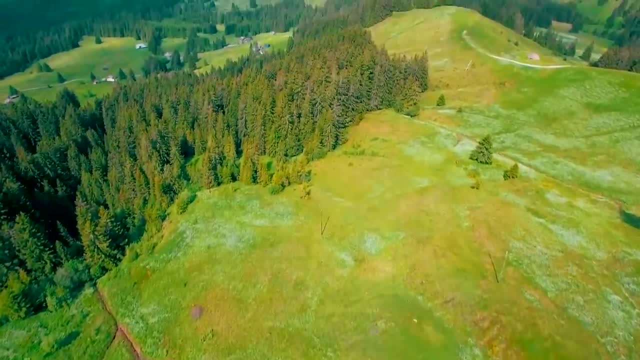 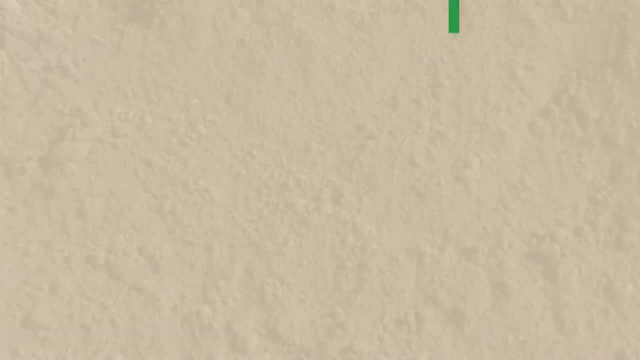 Based on the development of these layers, plus one or two other conditions, we can start to classify soils all over the world into soil orders. There are a bunch of these, so you better strap in So in the beginning, when there's soil with absolutely no development of horizons. 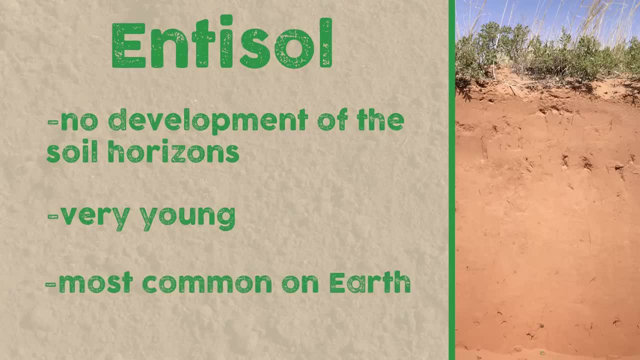 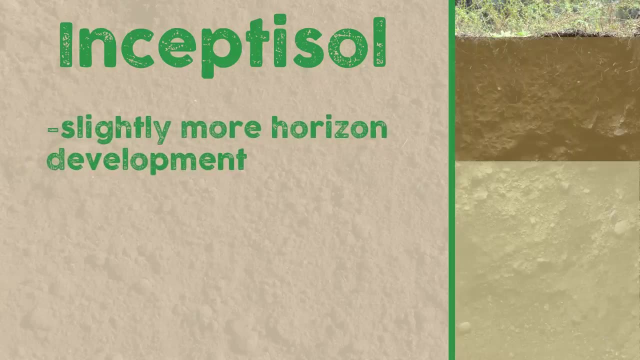 it's an entosol. These are very young and actually the most common type of soil on Earth. Give the soil a little more time, however, and it will become an enceptosol which has slightly more development of its layers, with the beginnings of a, B. 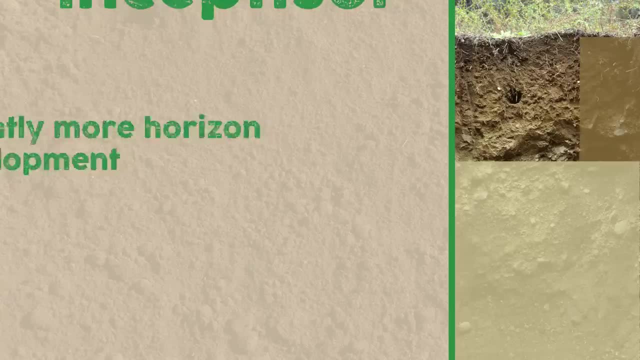 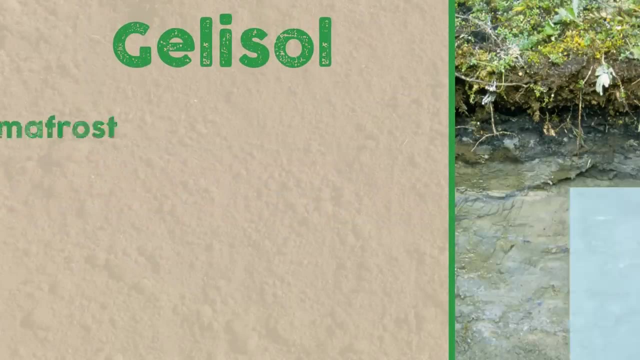 horizon. Then, based on the climate, given more time, an enceptosol can become a variety of different soils. At high latitudes, in the Arctic or even mountain ranges, you'll have gelisols. These soils will have permafrost close to the surface, so the soil doesn't move around a lot. 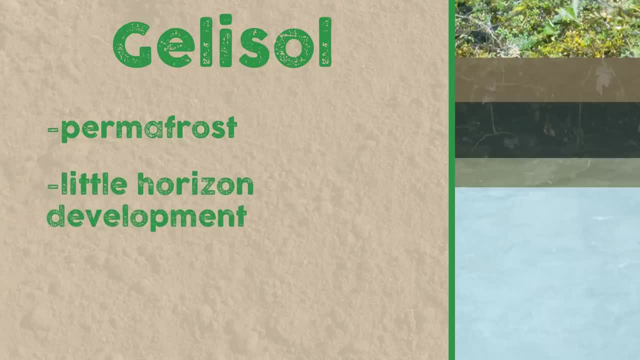 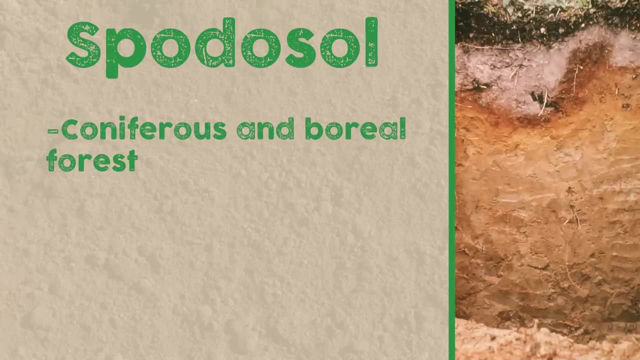 meaning its horizons remain undeveloped as well. These are found mostly within northern Russia and Canada. Moving slightly closer to the equator, we'll next find spotosols, which occur in coniferous and boreal forest biomes. These will be acidic, due to pine needles falling to the ground and decomposing into acidic compounds. 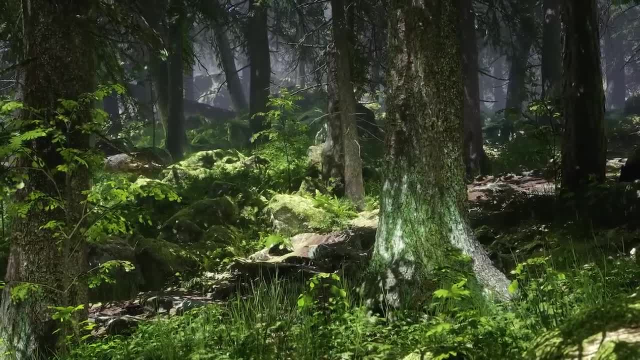 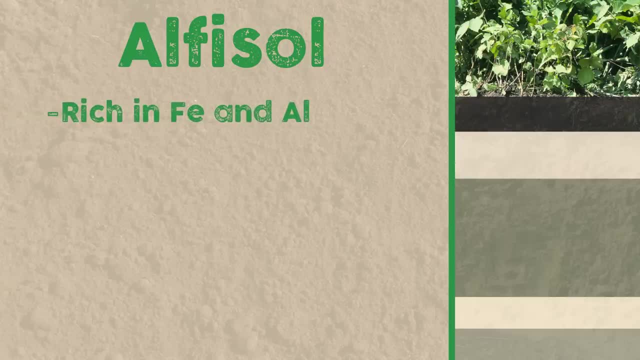 Because of this, they're low in fertility. These are primarily found in Scandinavia and the Canadian east coast. Then we have alphasols, which have fair horizon development. They're rich in iron and aluminum and are typically under broadleaf and deciduous forests. 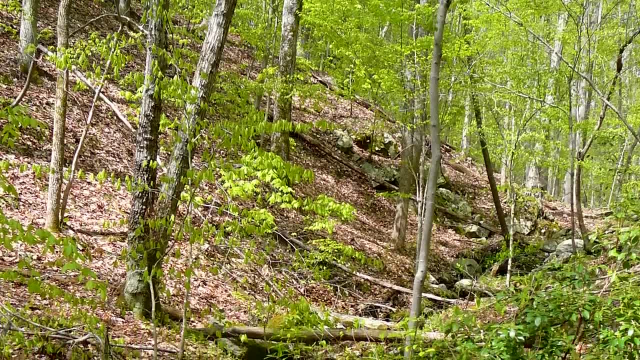 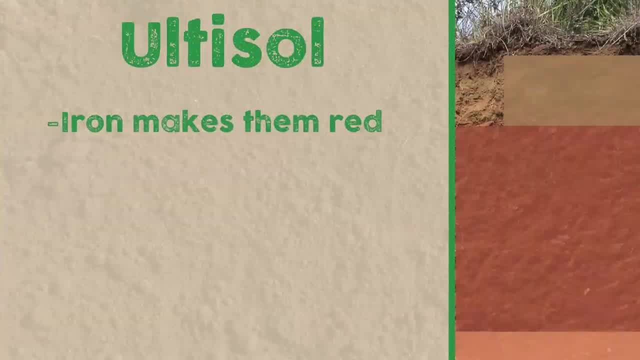 and also some human Mediterranean climates. These are mostly in the east coast of the United States and the Russian heartland. Below alphasols you'll have oltosols which have a lot more iron in them, making them very red. These occur in subtropical locations, very humid places like the American southeast and southeast Asia. 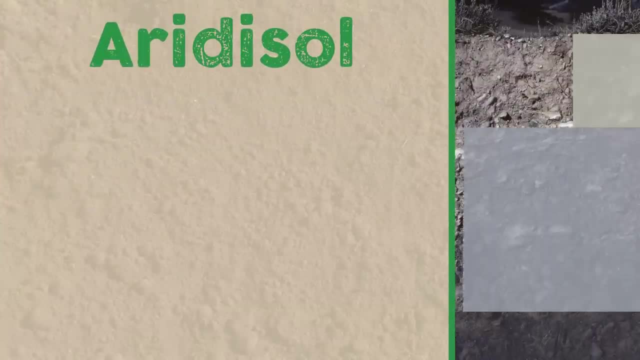 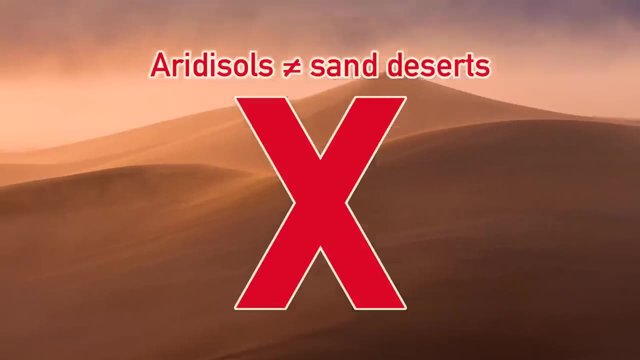 On roughly the same plain are iridesols. While oltosols occur in very humid places, iridesols are desert soils with extremely low amounts of water. Just think arid iridesols. These are not sand deserts, however. This is what an iridesol looks like and this is shifting sand. They're different. 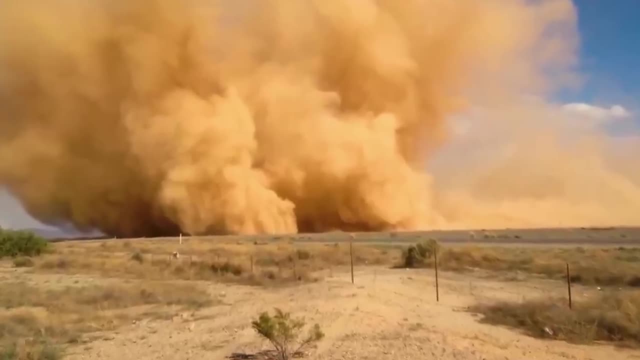 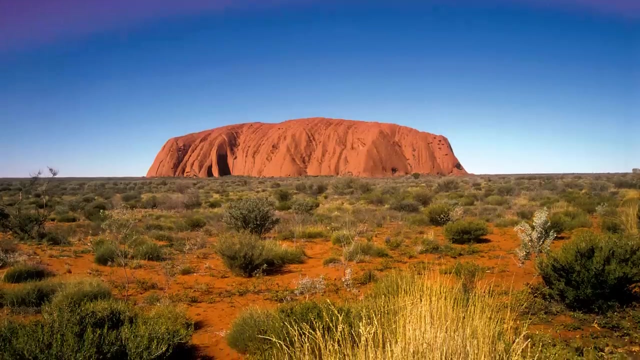 Because there's little to no water in these environments. most of the small clay particles have been blown away by the wind, leaving mostly heavier sand, silt and gravel. These are found in the Sahara, Arabia, Australia, northern China and the western United States. 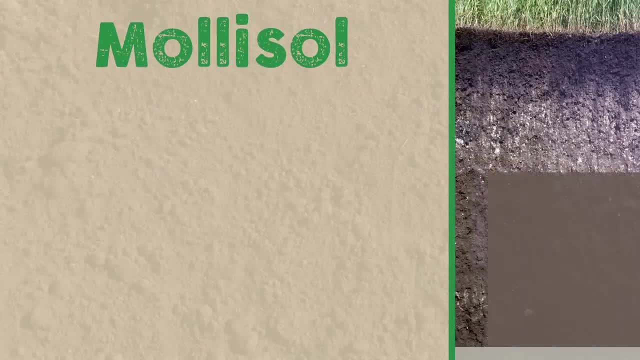 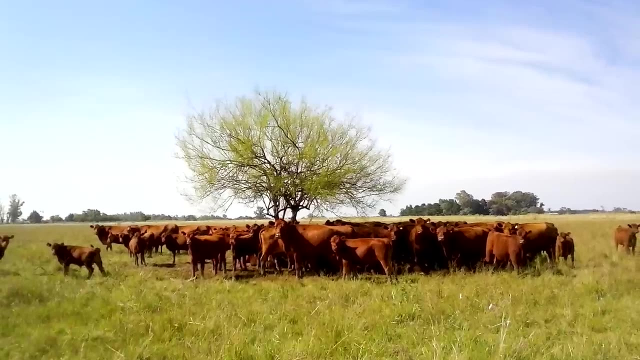 Also roughly in this area are mollisols. These are dark soils and, in terms of agriculture, the most fertile soil order. These occur in grassland regions like the American Midwest, the Pompous region of South America and the steppe region of Russia. 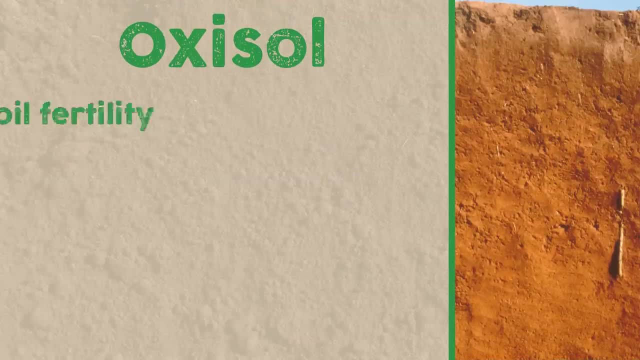 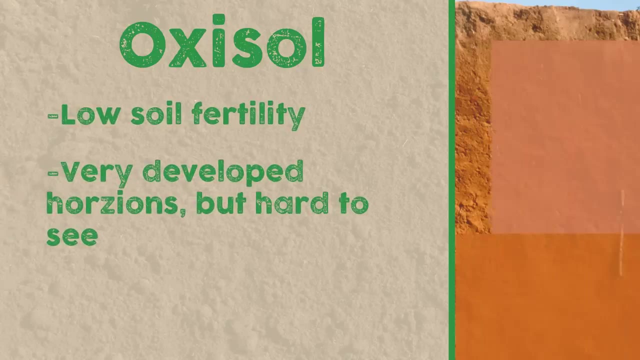 Lastly, in terms of latitude, we have oxisols. These have low nutrient availability and aren't very fertile, but they do have the most horizon development of any soil order. although it's hard to see because there's so much iron in the soil, turning every layer this reddish-orange color. 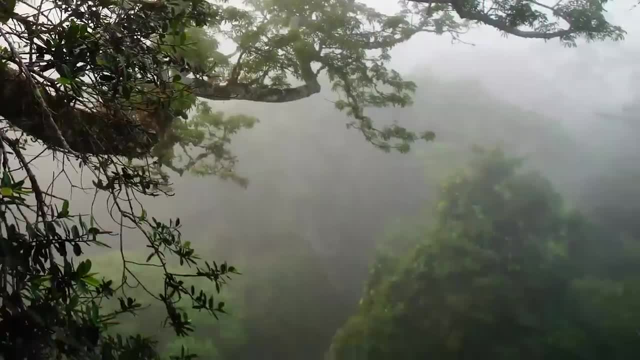 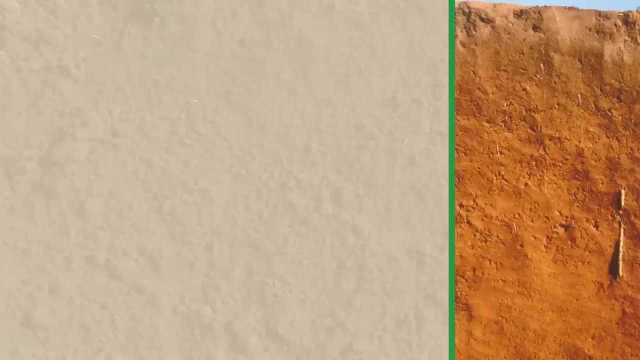 These are rainforest soils, Amazon and the Congo. Then we have a few more soils that don't really fit into the latitude scheme. These sort of just occur where they occur In this vague category. first you'll have andesols, Think like the volcanic Andes Mountains. 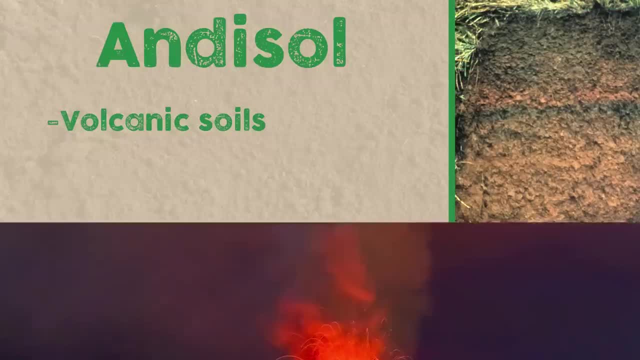 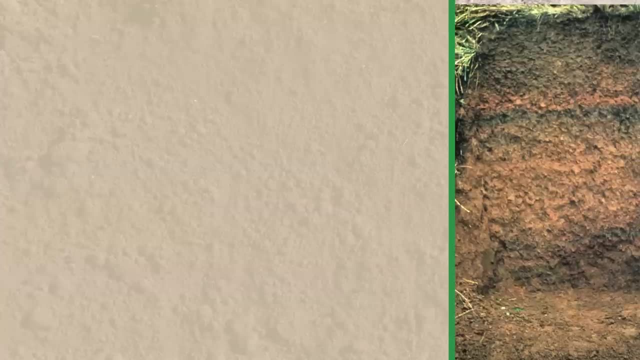 This is recently volcanic soil ejected from a volcano. These are surprisingly rich in nutrients and, given enough time, create lush landscapes. Think about the volcanic islands of Hawaii and Japan. Then we have histosols. These are wetland soils. That means they're caked in water and usually feature peat. 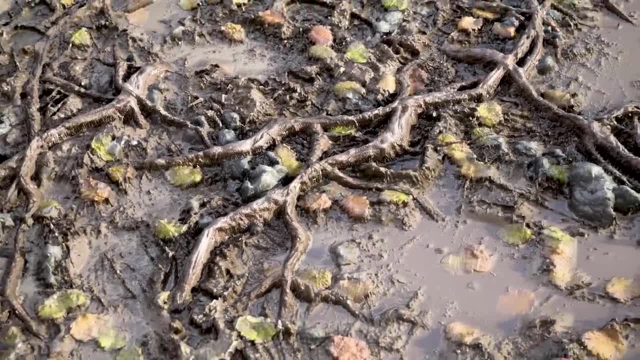 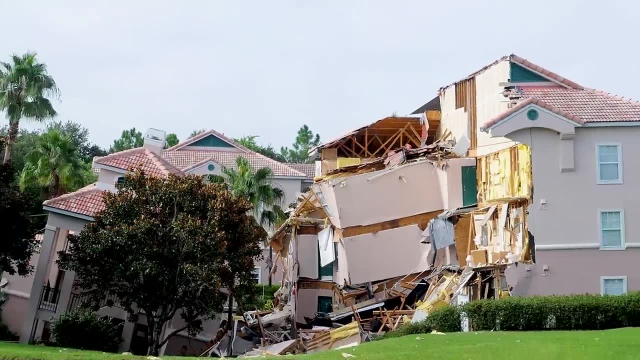 There's also going to be a lot of undegraded organic matter which can form an impermeable layer if too much builds up. Due to the buildup of this organic matter, these will also be highly acidic. They're also unstable and dangerous to build structures on. 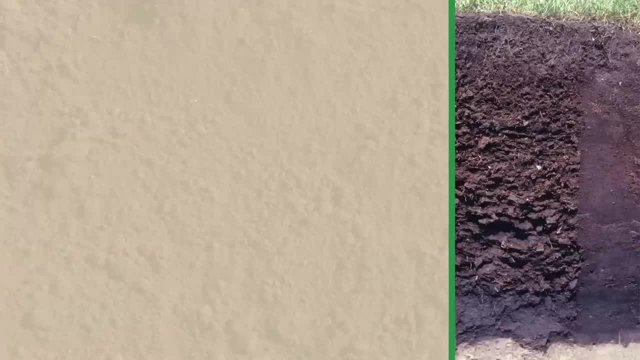 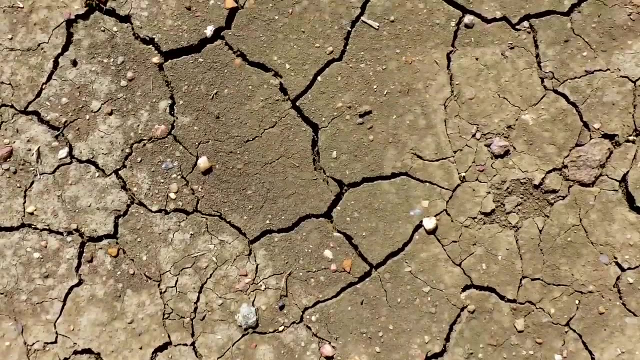 Most of these can be found in Canada and river deltas. And lastly, we have vertisols. These also have a lot of clay in them, but they often dry out. When they do, the ground will crack and split and look like this: 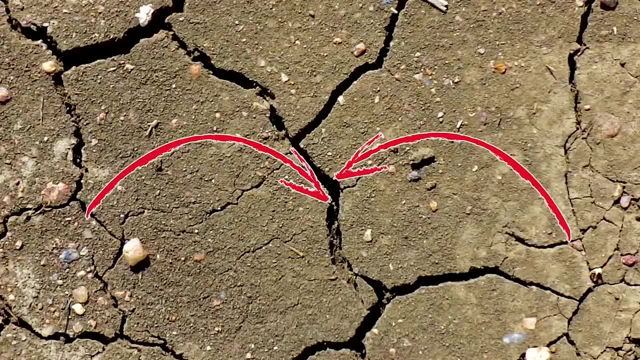 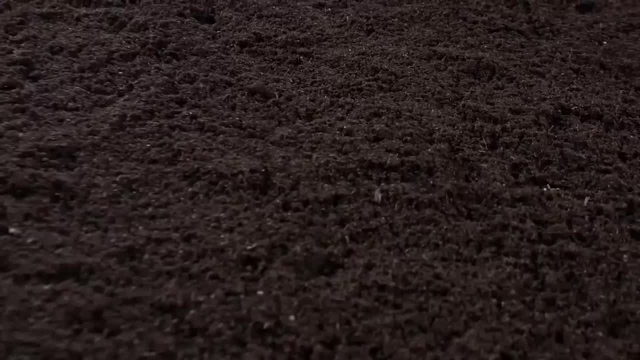 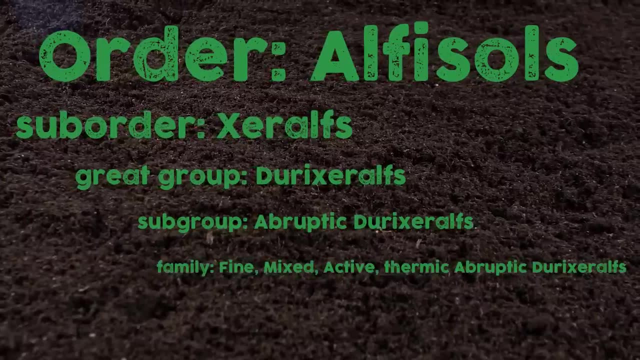 When this happens, soil on top will get blown into the crevices, inverting the soil layers and preventing real horizons from forming. The largest concentrations of them are found in India and Sudan. There are, of course, more ways to describe soil and, in fact, for every order there's a suborder, a great group, a subgroup, a family and a series. 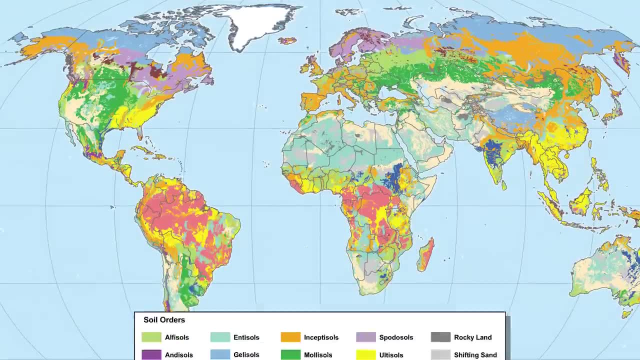 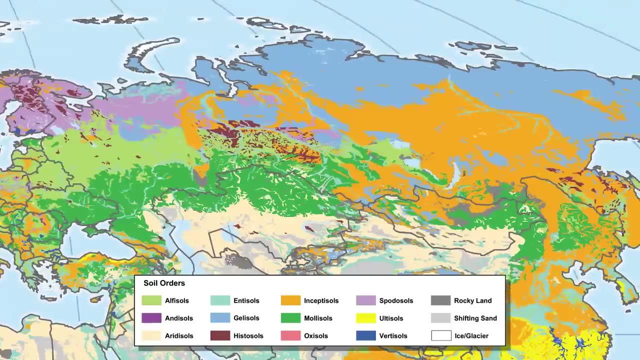 But, holy crap, we don't have enough time for that. Here's a map of the actual distribution of these soil types across the planet. You'll see most of the new soils are close to the poles. This is because, until recently, the poles were covered in glaciers from the last ice age, so they haven't had much time to develop. 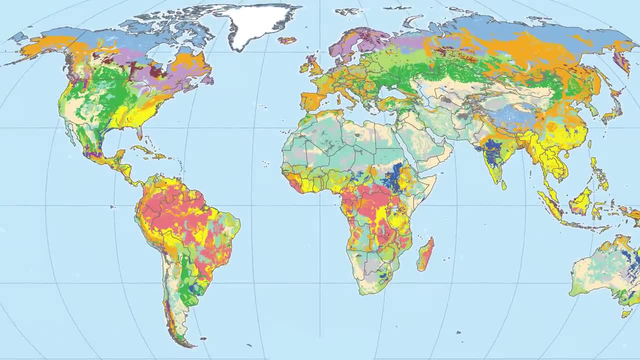 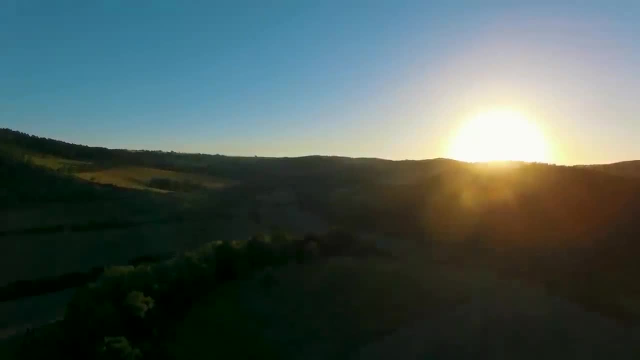 I'll leave a link for a bigger version of this map in the description. But the soil distribution is kind of sporadic and patchy, and that's because latitude and humidity aren't the only things that determine where different orders of soil are found.